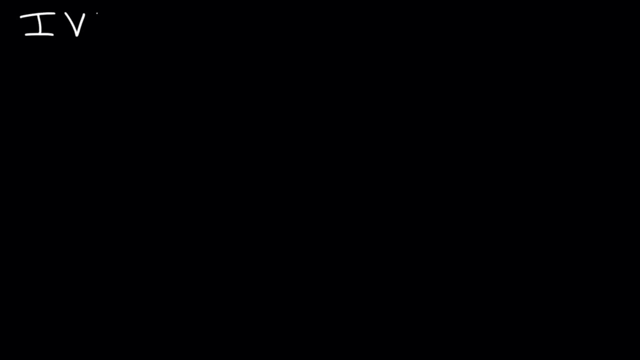 Now let's talk about IVT, the intermediate value theorem. The intermediate value theorem states that if f is continuous on a closed interval, a to b and f of a does not equal f of b, and k is any number that's between f of a and f of b. then 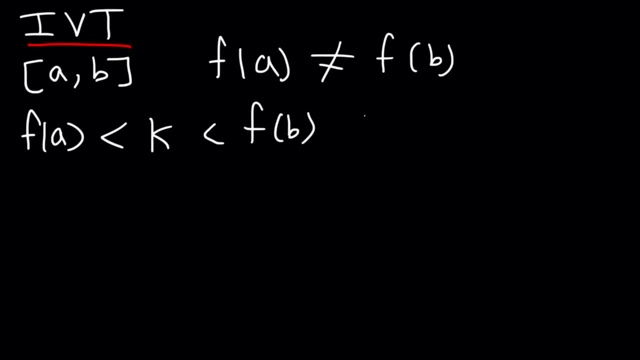 there's at least one number c on the interval a to b, such that f of c is equal to k. Now let's go ahead and apply this information. So how can you use the intermediate value theorem to show that there's a root or zero in this function within the specified interval, where the interval is? 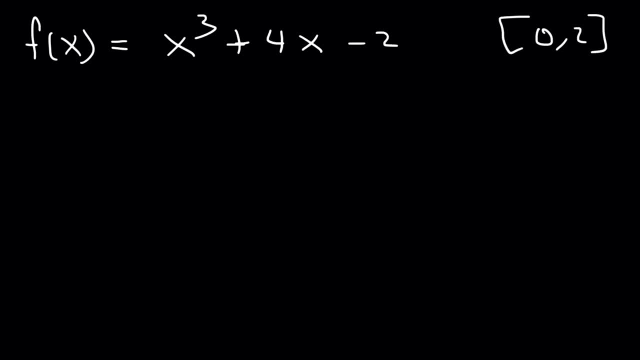 from 0 to 2?. How can you use the intermediate value theorem to prove that? Go ahead and try So. first we need to find the value of f of a and f of b, in this case f of 0 and f of 2.. a is 0, b is 2.. 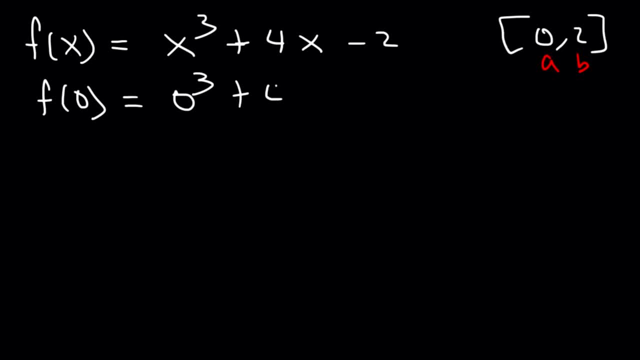 So f of 0 is going to equal negative 2.. Now let's find the value of f of b or f of 2, which is 2 to the 3rd plus 4 times 2 minus 2.. 2 to the 3rd is 8, 4 times 2. 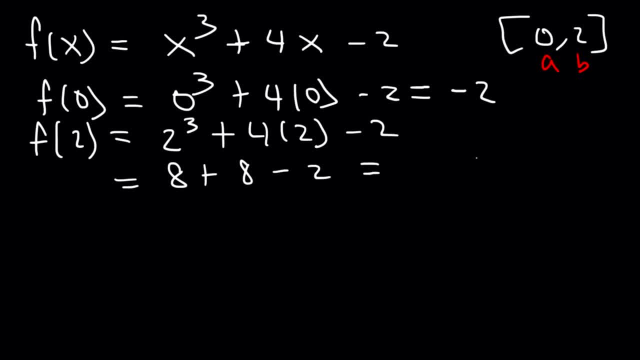 is also 8.. 8 plus 8 is 16, minus 2, that's 14.. So f of a is negative 2, f of b is 14. now keep in mind: K is between F of a and F of B, so K is between negative 2. 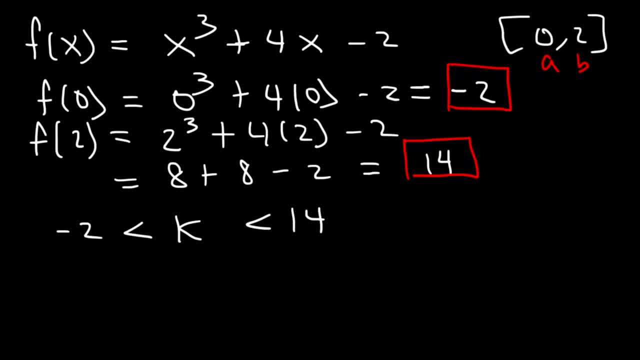 and 14, and our goal is to show that there is a root or a number that's equal to 0. so we got to show that there's some value C where K is 0 and 0 is between negative 2 and 14. so there is some value out there where K can be 0 because 0. 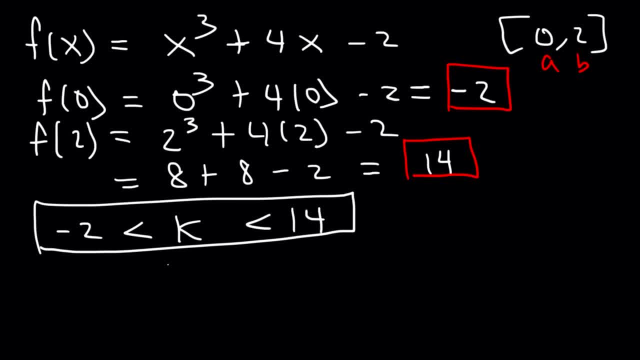 isn't within its range. so if you think about it, if we have some function where F of 0 is negative 2 and F of 2 is 14, so that's probably way up here, and if it's continuous at some point, let me draw a better line. at some point the curve has to cross the x-axis, so 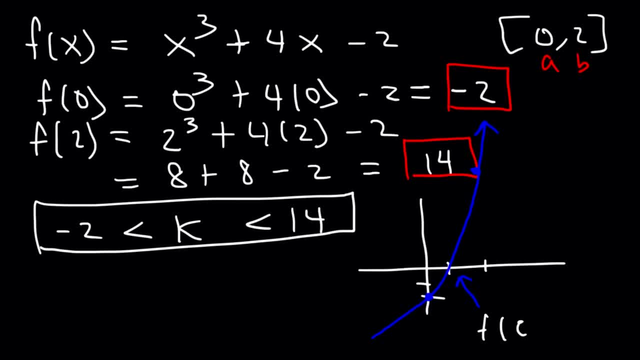 there's some value where F of C is equal to 0, and keep in mind, F of C is K, so there's some value where K is equal to 0, so it's going to be a root or 0 in the equation. in order to find it, we need to set F of X equal to 0, and then we could. 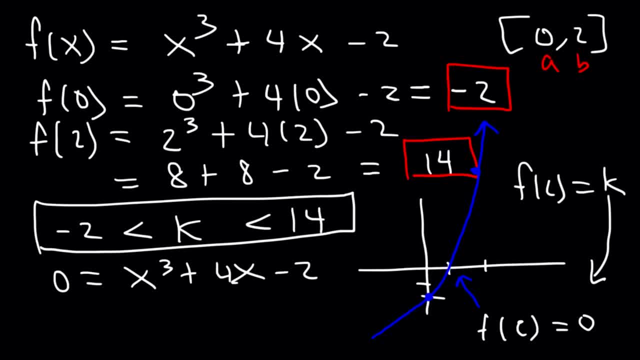 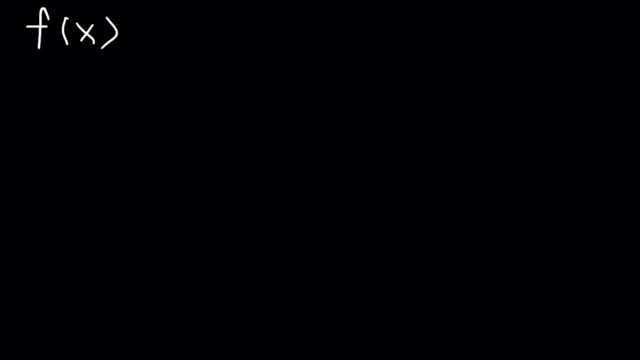 solve the equation for x. we know it's somewhere between 0 and 2. it's not 1 because if we plug in one we're going to get positive 3. so technically it's going to be between 0 and 1. let's try a different example. so let's say that F of X is equal to x squared. 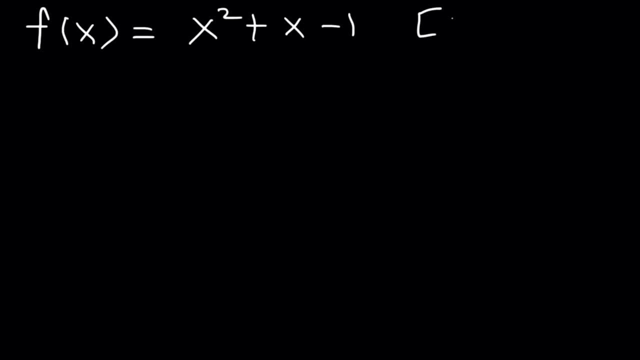 plus X minus 1 on the interval 0 to 5, and that F of C is equal to 11. so the instructions are going to be different from the last example: verify that the intermediate value theorem applies to the indicated interval and find the value of C guaranteed by the intermediate value theorem. so first we 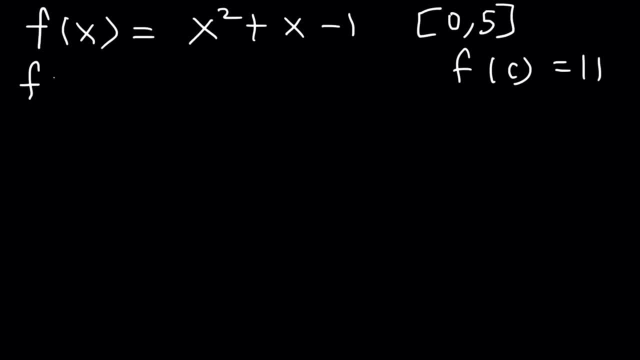 got to make sure it applies to the interval. so we get to find F of A and F of B. so F of 0 is 0 squared plus 0 minus 1, which is negative 1. so that's F of A, F of B, and the answer is F of A minus one. so the answer is F of B. 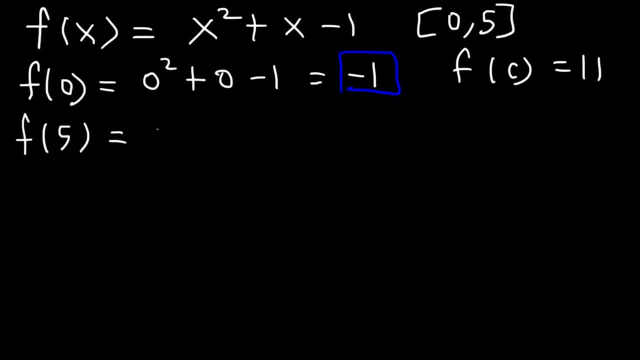 which is the same as f of 5, is going to be 5 squared plus 5 minus 1.. 5 squared is 25 plus 5, that's 30, minus 1, that's 29.. So that's the value of f of b. 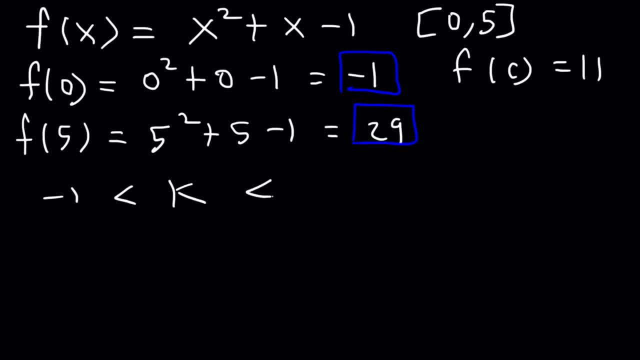 k has to be between negative 1 and 29.. Now keep in mind f of c is equal to k, So therefore k is 11.. So 11 is between negative 1 and 29.. So the intermediate value theorem does apply to this function within this interval. 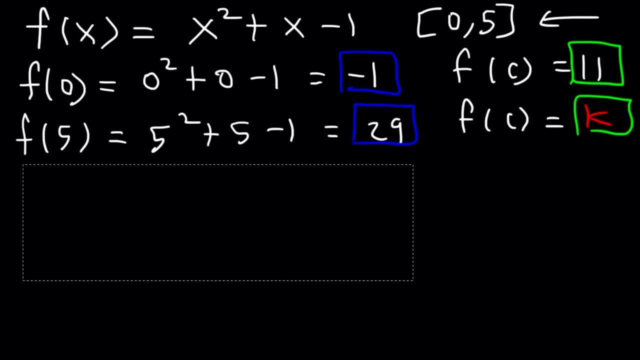 So now we've got to find f of c. I mean not f of c, but the value of c. f of c is 11.. So we're going to set 11 equal to the function f of x And find the value of x. 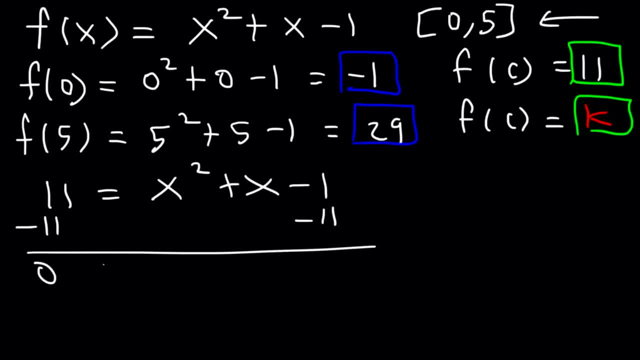 So let's subtract both sides by 11 to begin with. So x squared plus x minus 12 is equal to 0.. So now we can factor. We need to find two numbers that multiply to negative 12, but add to the middle coefficient of 1.. 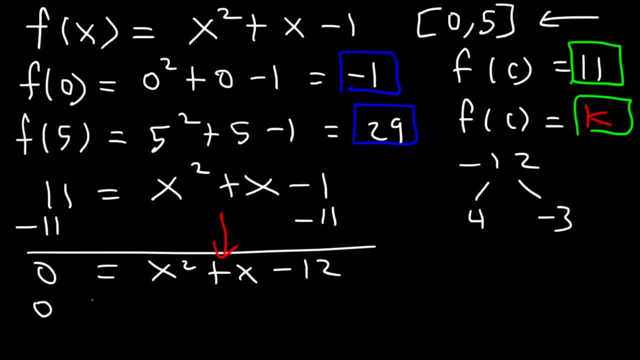 So this is going to be positive 4 and negative 3.. So therefore, we're going to have x plus 4 and x minus 3.. So we can see that x is equal to negative 4 and positive 3.. So now, which x value? 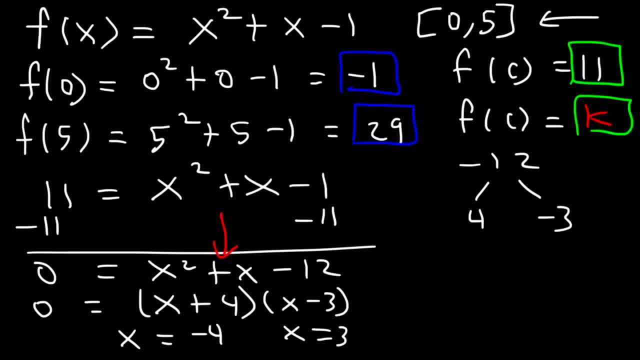 Is the actual value of c? Is it negative 4? Is it positive 3? Or is it both? Now we need to find out which one is in the interval. Negative 4 is not between 0 and 5. But positive 3 is between 0 and 5.. 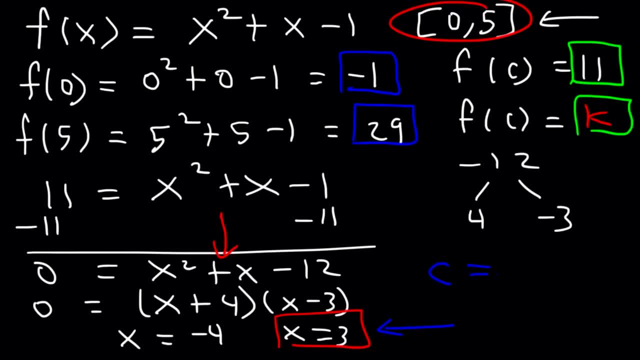 So c is equal to this particular x value. So c is equal to 3.. f of 3 is 11.. And 3 is In the interval. It's between a and b. So this is our answer: c is 3.. 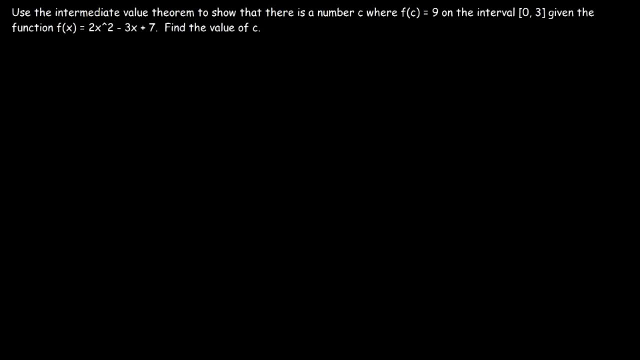 Here's a problem that you can work on. Use the intermediate value theorem to show that there is a number c where f of c is equal to 9 on the interval 0 to 3.. Given a function, f of x is equal to 2x squared minus 3x plus 7.. 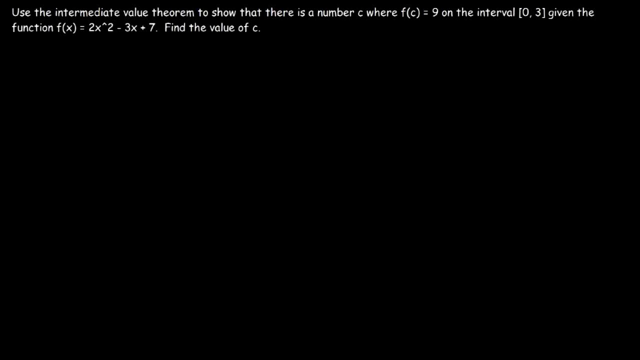 In addition, find the value of c. So first Let's evaluate the function at a and b. So let's find the function value when x is 0. So let's plug it into that equation. So it's going to be 2 times 0 squared minus 3 times 0 plus 7.. 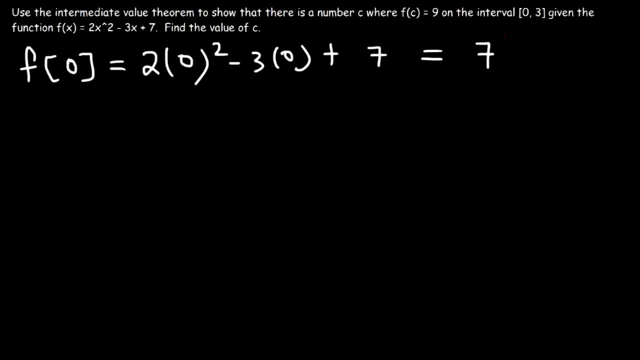 So that's equal to 7.. Now let's evaluate the function when x is equal to 3.. So it's 2 times 3 squared minus 3 times 3 plus 7.. 3 squared is 9, and 2 times 9 is 18.. 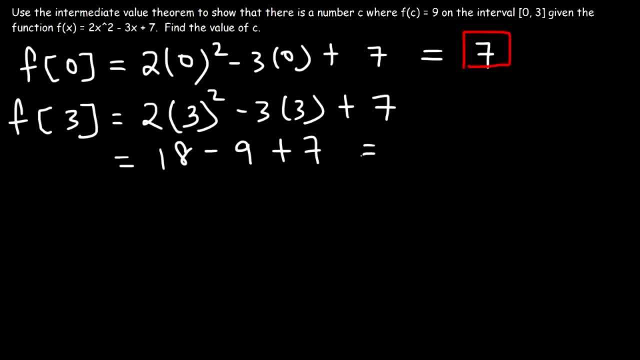 3 times 3 is 9.. And then 18 minus 9 is 9.. 9 plus 7 is 16.. Now Now f of c is equal to 9.. And 9 is basically the k value. 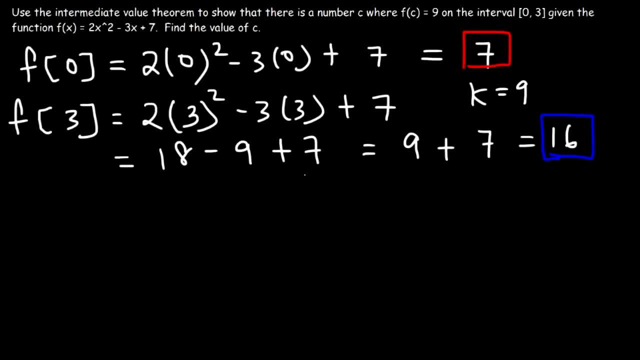 So we can say k is 9.. So notice that k or 9, is between 16 and 7.. Therefore c, which is an x value, has to be between a and b, So c is between 3 and 0.. 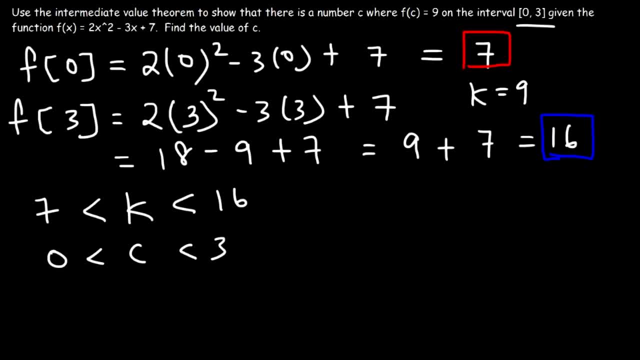 Now let's go ahead and calculate c. So let's set the function to be equal to k or 9.. So 2x squared minus 3x plus 7 will be set equal to 9.. So if we subtract both sides by 9, 7 minus 9 is negative 2.. 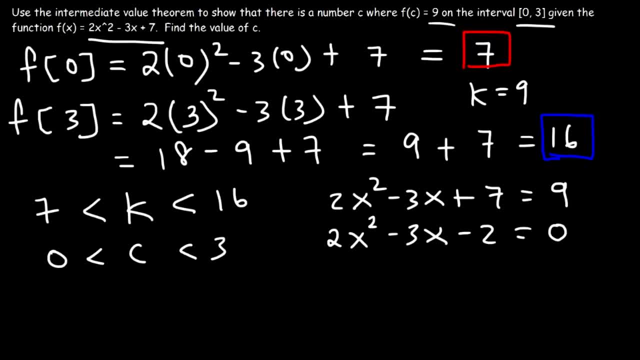 So we're going to have negative 2 on the left side. Now we need to factor this trinomial And the leading coefficient is not 1, it's 2. So we need to multiply the leading coefficient by the constant term. 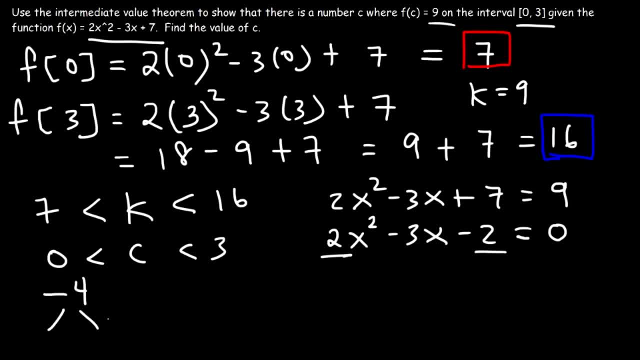 2 times negative. 2 is negative 4.. And we need to find two numbers that multiply to negative 4, but add to the middle coefficient negative 3.. So that's negative 4 and 1.. Now we're going to replace negative 3x with negative 4x plus 1x. 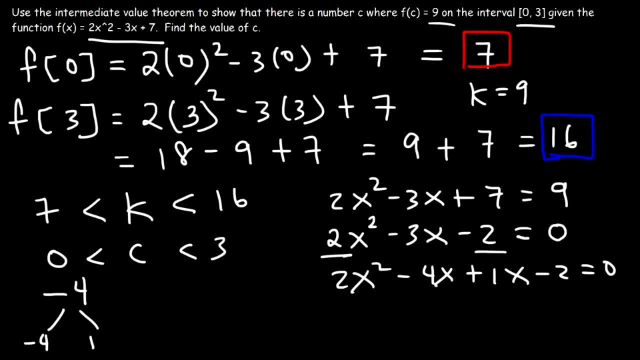 And then factor by grouping. So in the first two terms, take out the GCF, which is 2x. 2x squared divided by 2x is x Negative. 4x divided by 2x, that's going to be negative 2.. 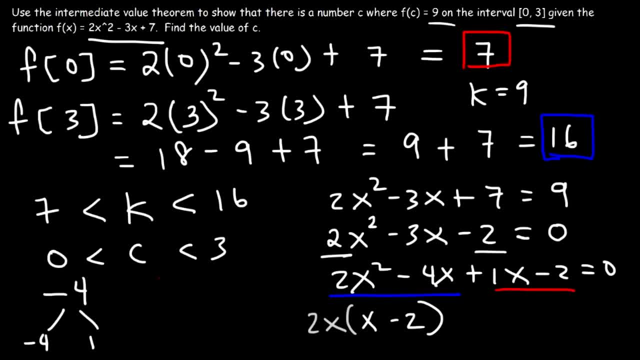 Now, in the last two terms, there's nothing to take out. So take out a 1.. If we take out a 1, we're still going to get x minus 2.. Now we need to factor the greatest common factor again.